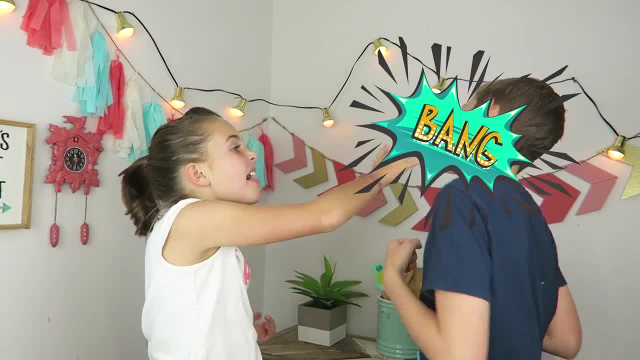 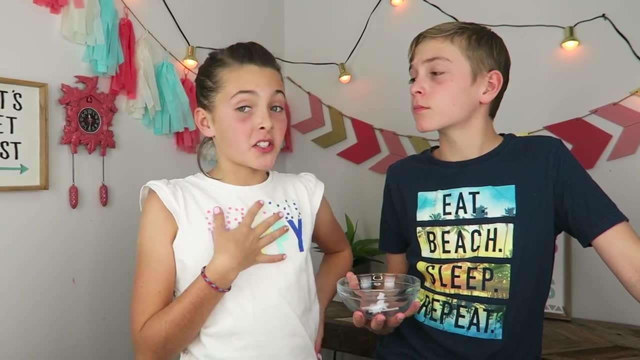 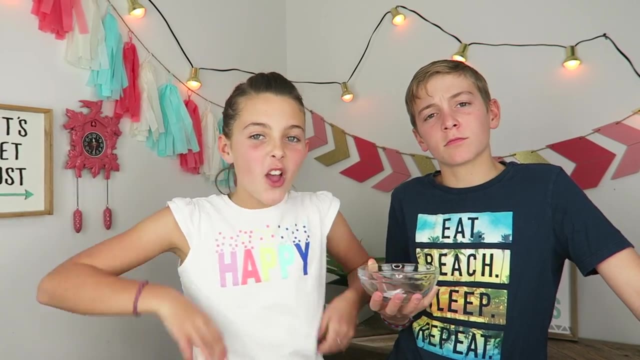 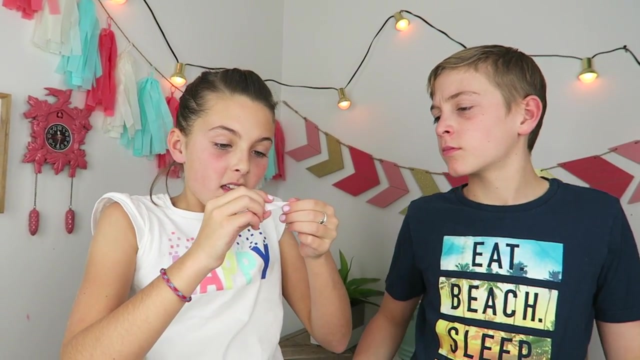 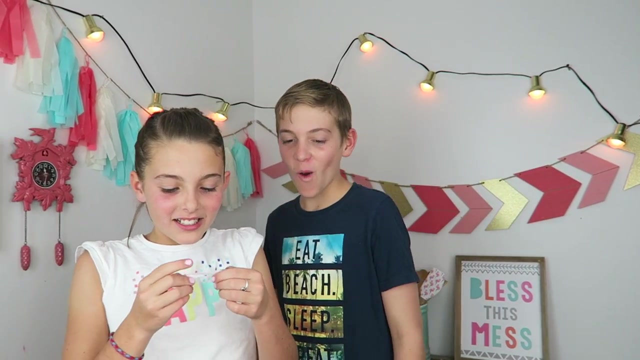 Okay, let's get started. I'm gonna draw first, but before we do, don't forget to subscribe and turn on notifications, So you know when we upload a new video, Cornucopia what is that? It's okay, She doesn't know. that means I'll win. 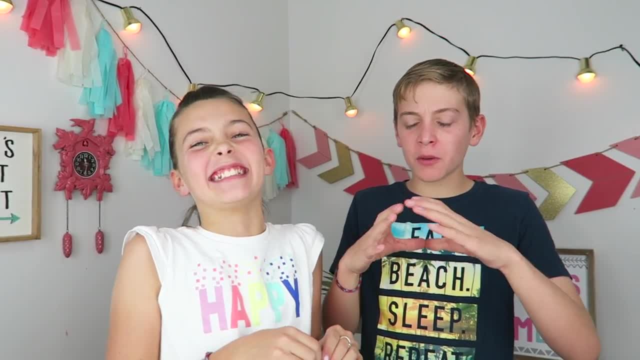 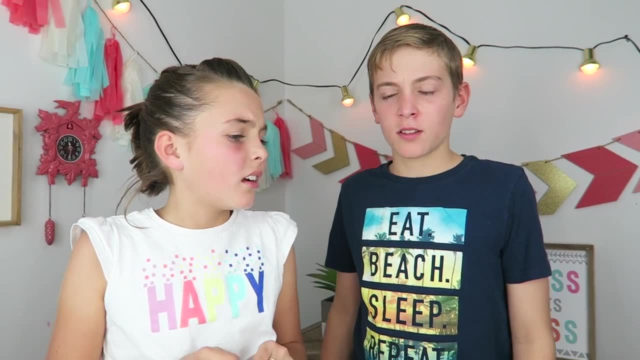 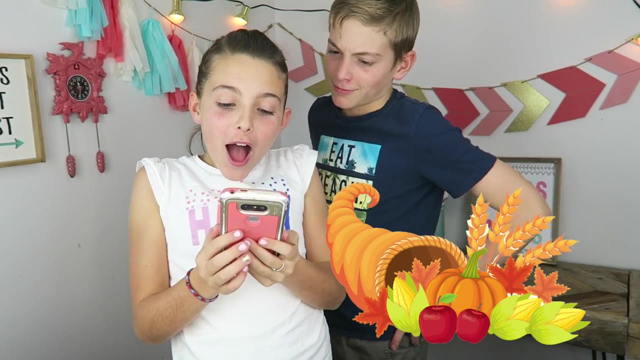 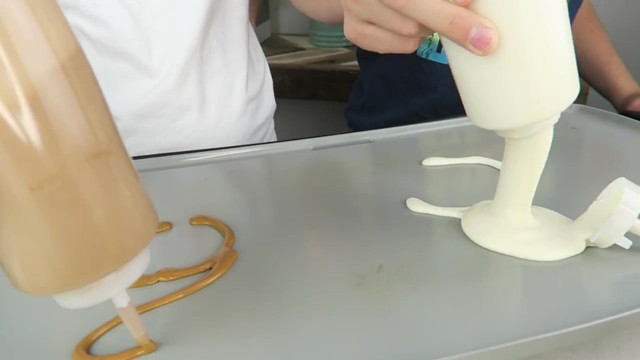 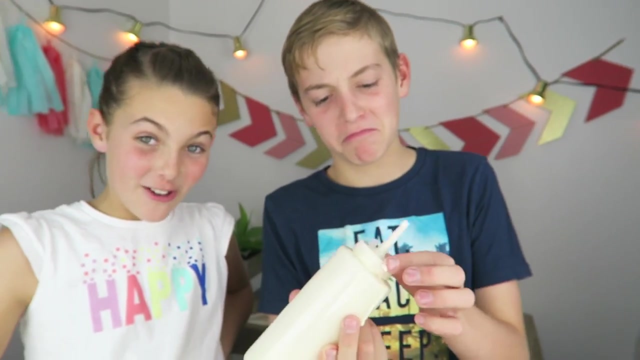 Cornucopia. Cornucopia is like, it's like it looks like a bull's horn, but it's like hollow and they like put stuff in it. Okay, let's do this thing. Oh my gosh, Malfunction, you guys. the lid popped up and it just exploded. I'm going to win. 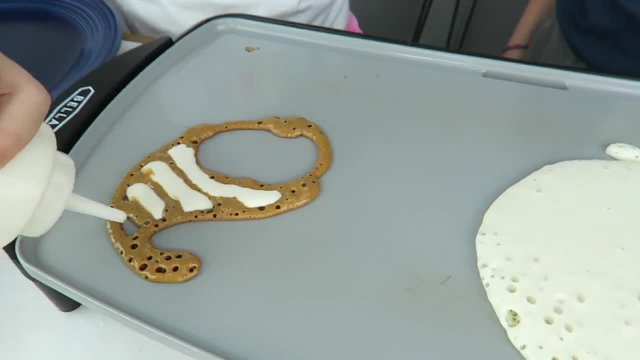 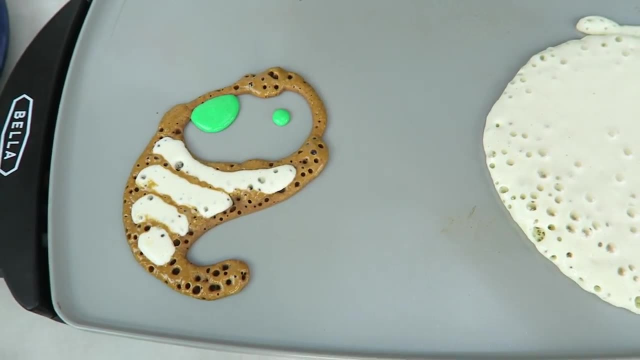 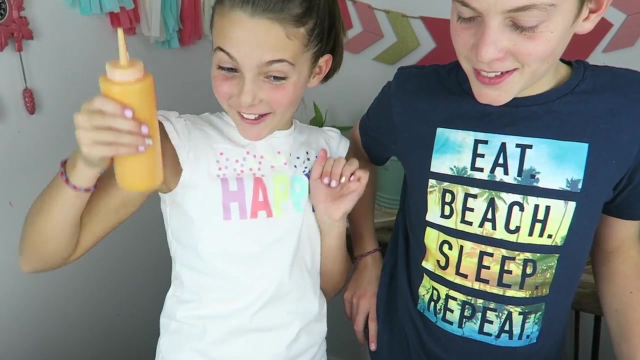 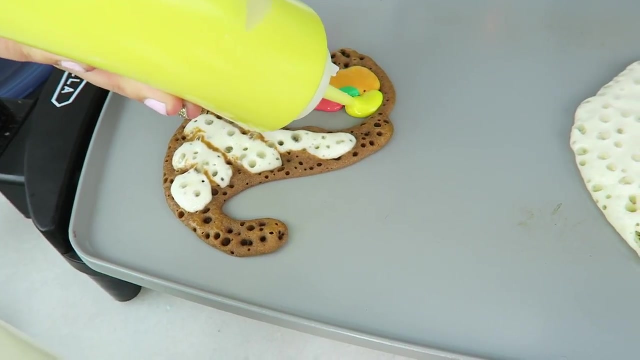 No, it's not fair. I'm going to draw a leaf here And then a stem right here, And then I'm gonna get this And I'm gonna draw a pumpkin- Oh, that's good- meanwhile Baking a normal pancake right here. That's a really good pancake. 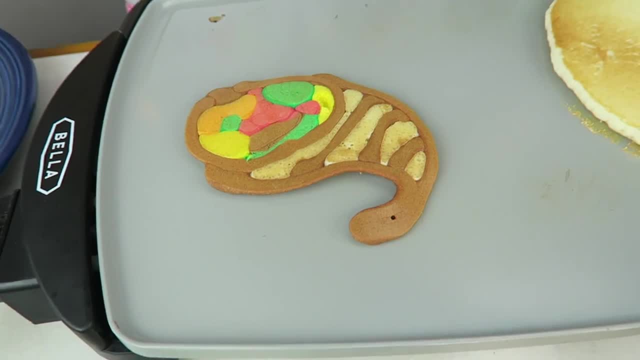 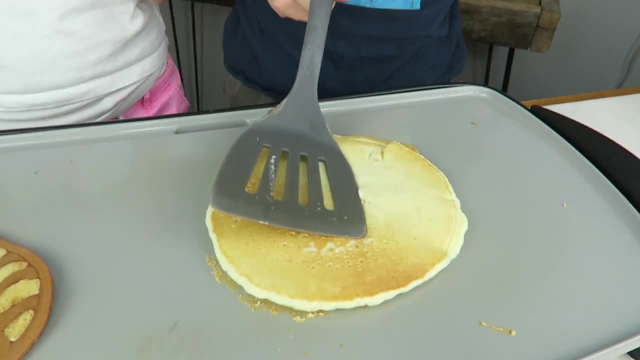 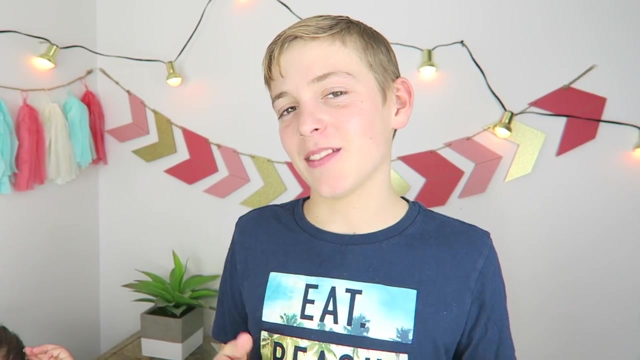 I was trying to make a pancake. Yay, It works. Yes, Na-na-na-na-na-ay, Na-na-na-na-na-ay. So I get to try again, because I had a little bit of technical difficulties. So yeah, Cornucopia. 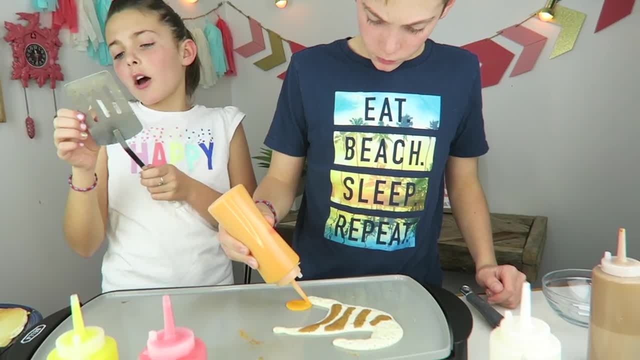 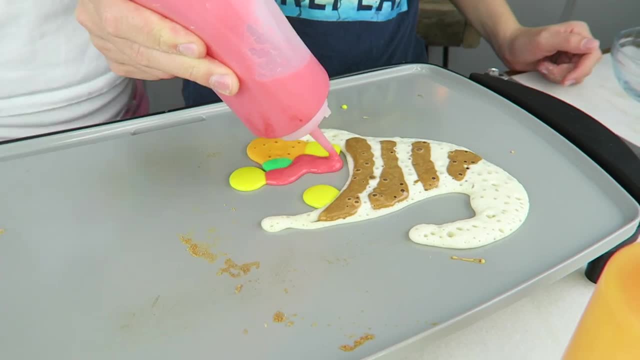 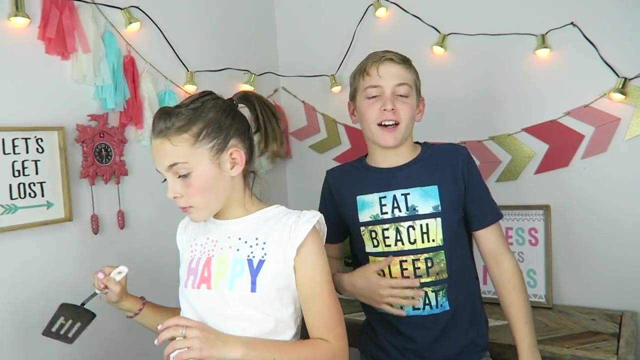 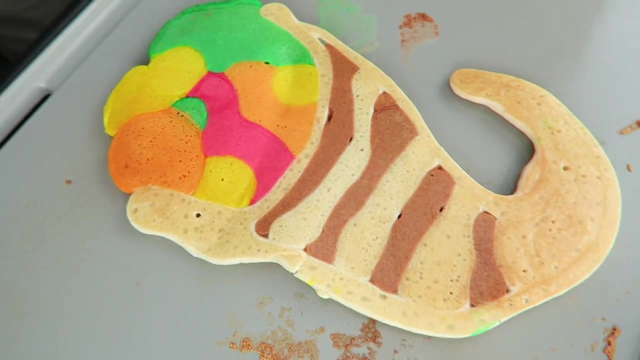 Cornucopia, It's a cornucopia. It's a Cornucopia. Ha, I am done with my Cornucopia. Yeah, Yeah, Cornucopia. That was actually pretty good. It looks more like cornucopia. 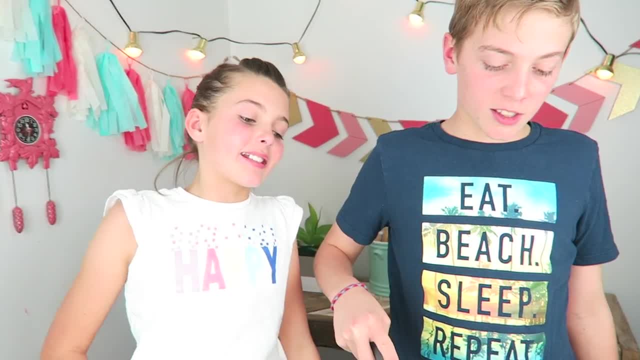 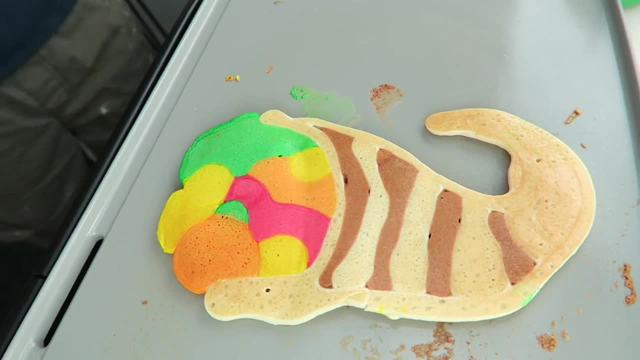 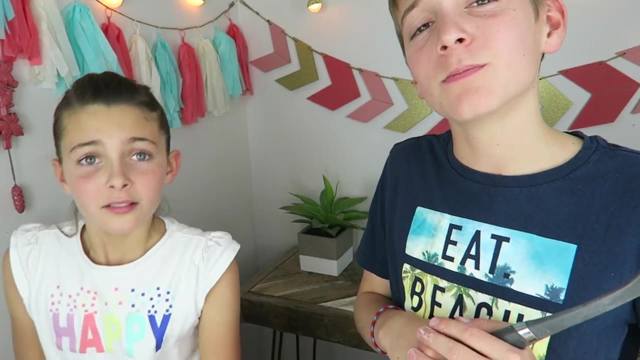 It's more like a giant like worm thingy That's eating vegetables. No, it's eating rainbows. It's a giant worm eating rainbows. Whose is better, Mine or Corbin's Mine? Comment down below. Comment down below My turn. 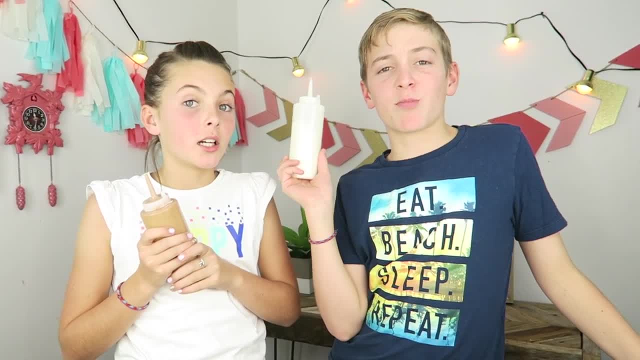 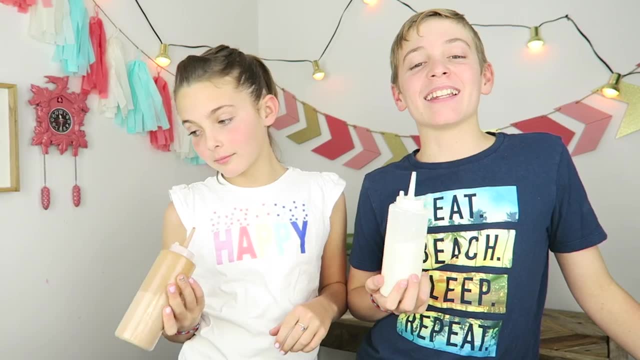 It is a turkey leg. You're liking the best part. I always like call dibs, like three hours a day, Dibs Before we eat. It's true, Before we eat it, because I don't want anybody else to take it, Because it's like the best part. 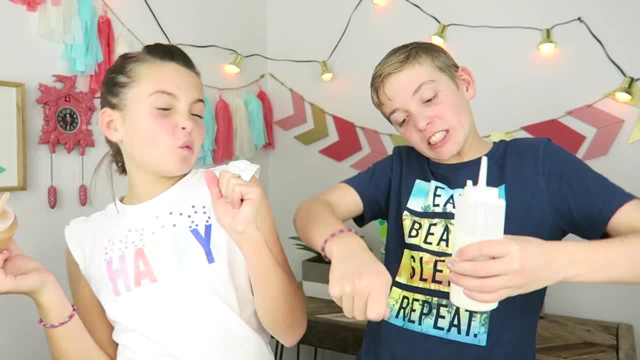 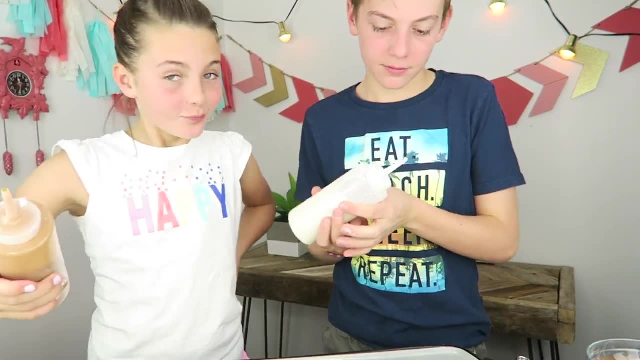 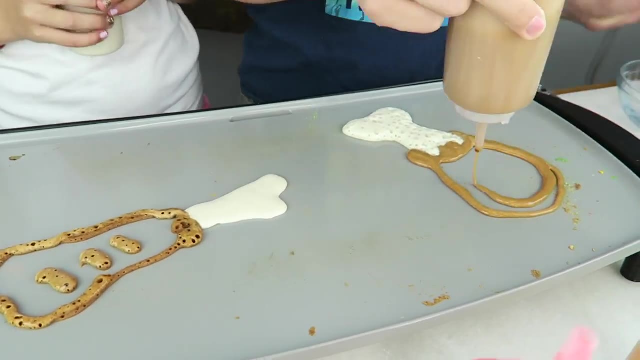 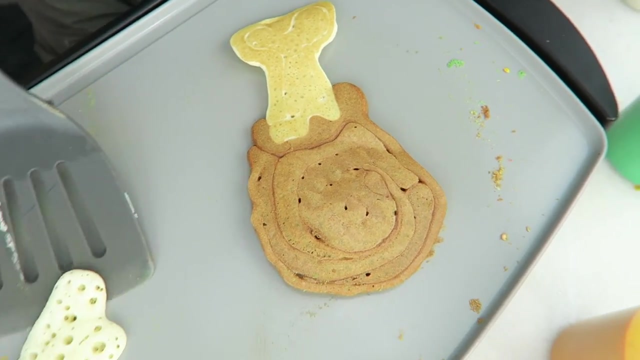 Because you can like, grab it, Like you don't have to use like a fork, and you're like, You're just like a caveman. Okay, let's get started. I already failed. I'm gonna break it. Corbin, can you help me? Can you help me with that? 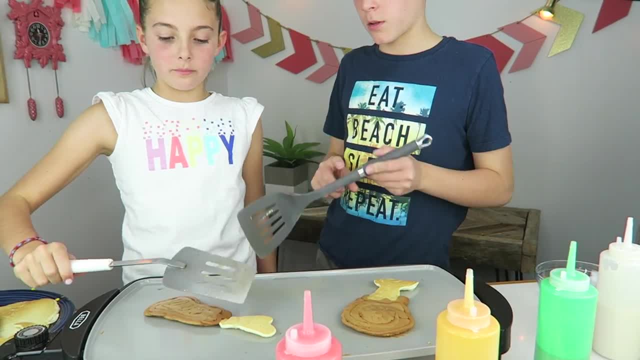 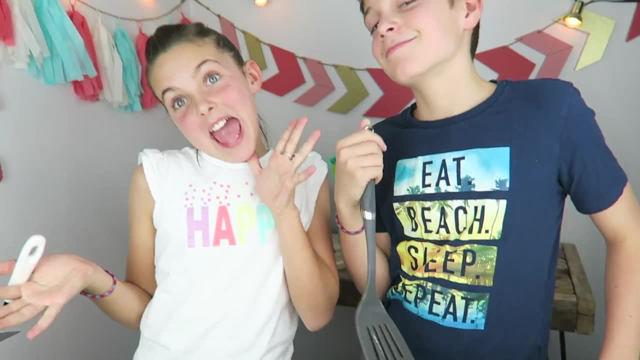 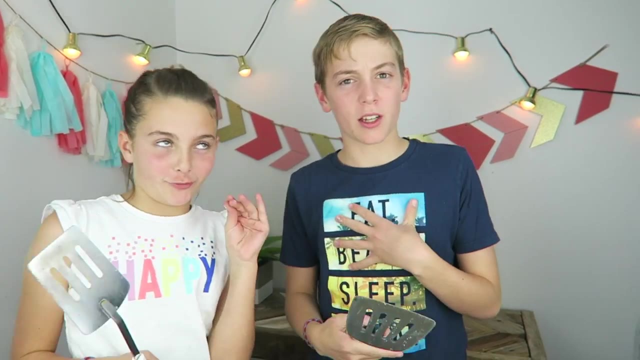 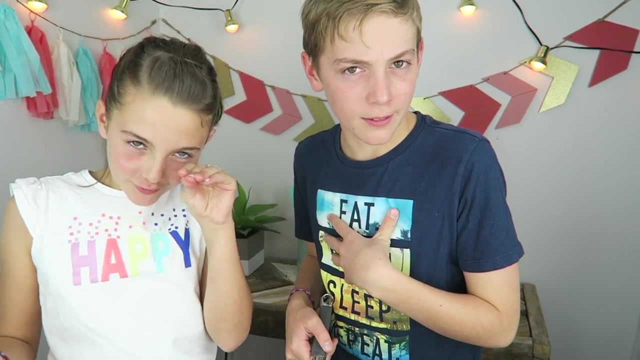 I'm gonna flip now There. Yeah, That was actually pretty good. We're finished. Yay, Corbin won turkey leg. okay, That's how you vote for me, because I'm the best at pancake art People. Seriously, Okay, guys, it's my turn. 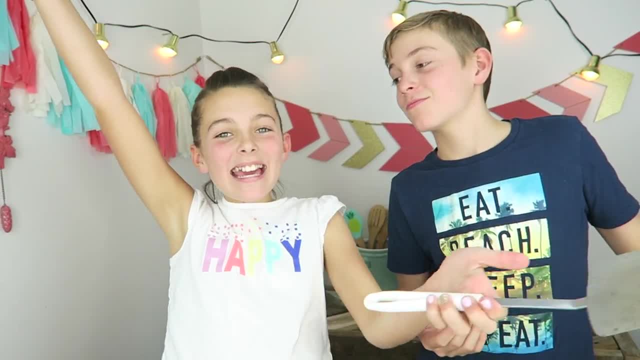 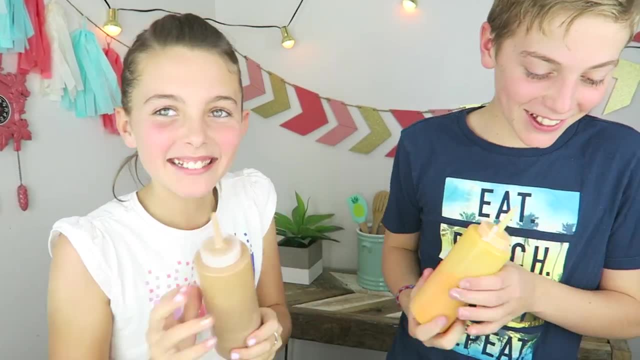 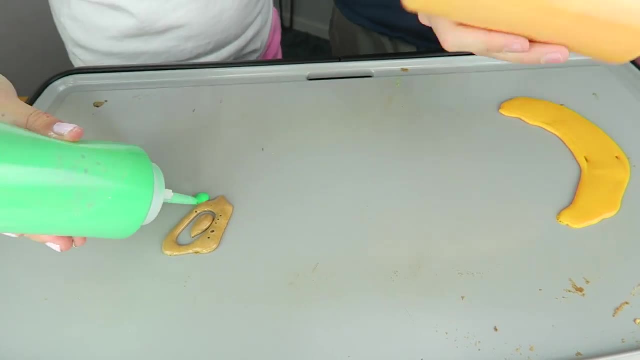 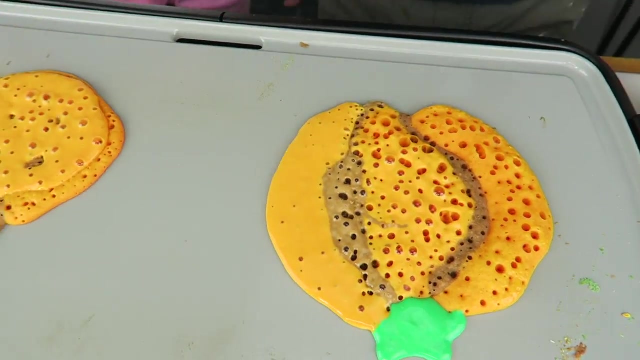 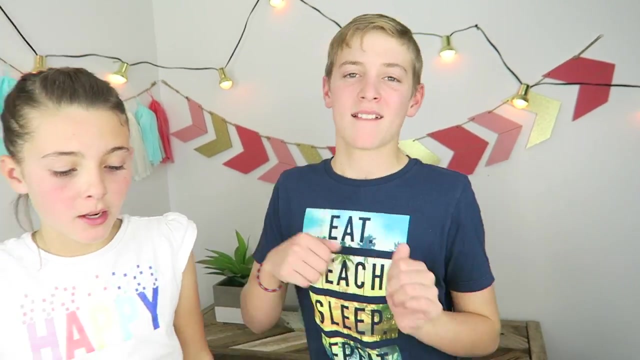 What is it? It's a pumpkin. Can I use that? because you're using the orange button? I need it. I'm using these. Nothing going on here, people And we're done. Pumpkin: Got my curlicues. at the end A bomb. Look how amazing that is. 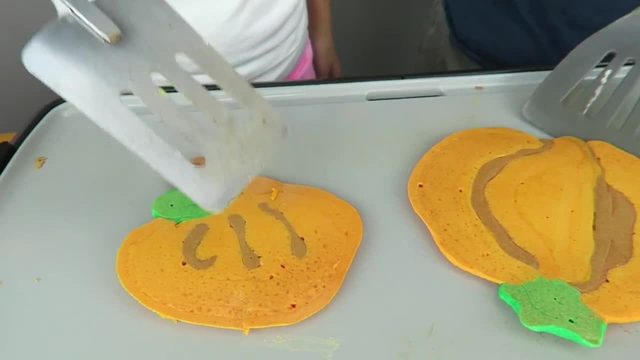 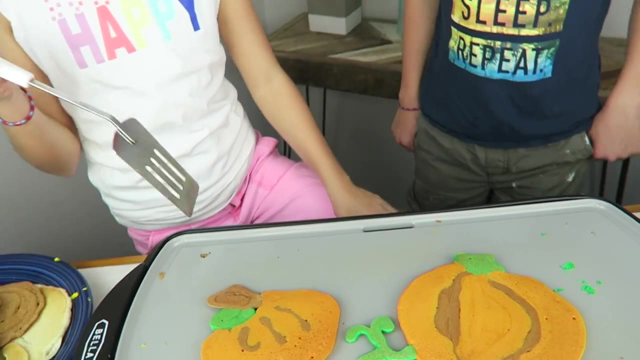 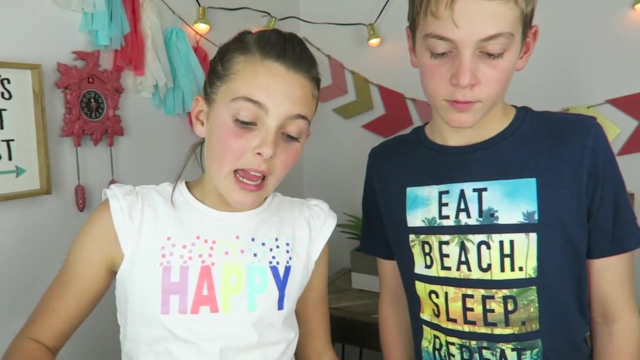 Does that look like a pumpkin? Okay, we're done. I tried to add a little bit, a little bit of detail in mine, Like I put the lines of the pumpkin, Like I tried to make a detail due to the stem of the pumpkin, But it didn't work. 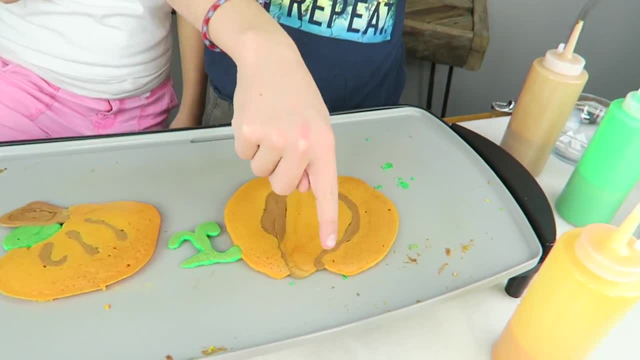 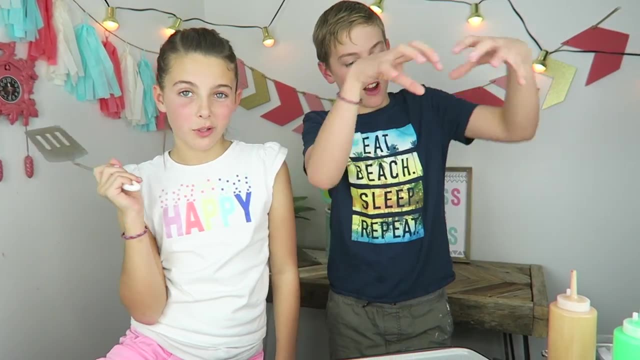 Because I didn't wait long enough, Like I tried to make it so that it looked like there was like a dip in And then the pumpkin came out. you know, That was a good idea. That's what I did. The vine thing is because pumpkins like grow on really long vines. 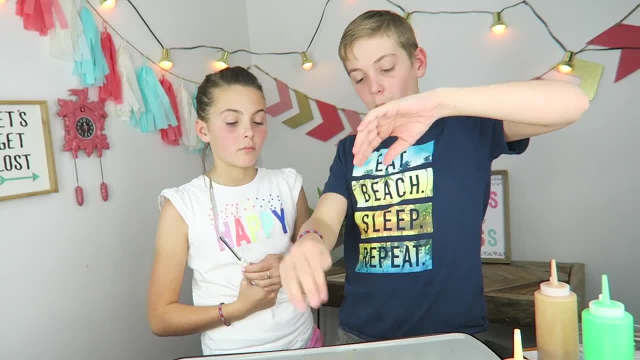 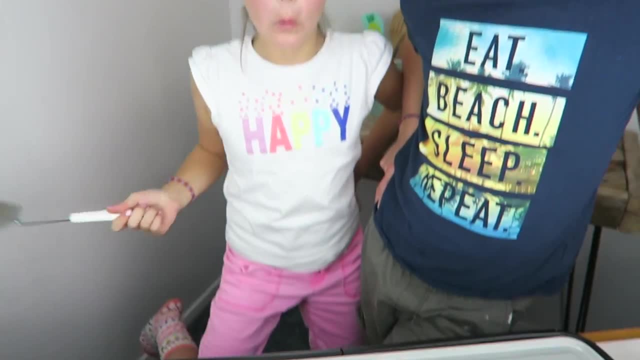 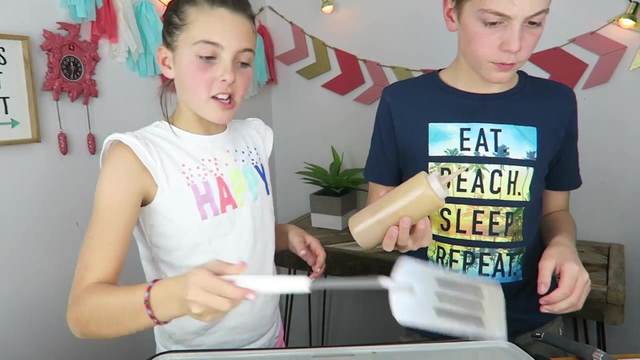 And they kind of just like spread out everywhere. So like I put a little one right here, Okay, guys, time to vote Mine or Corbin's Comment down below. What is it? Pumpkin pie, Woo, Okay, I'm planning it in my head, I'm just gonna go. 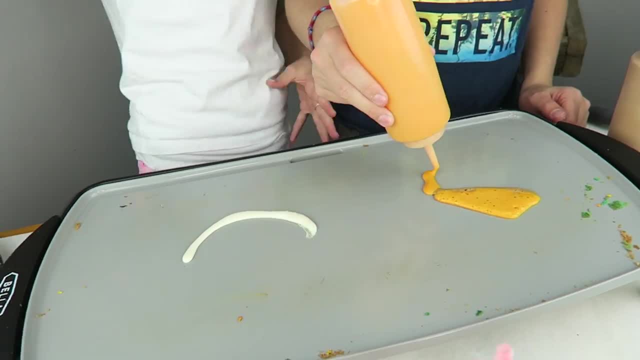 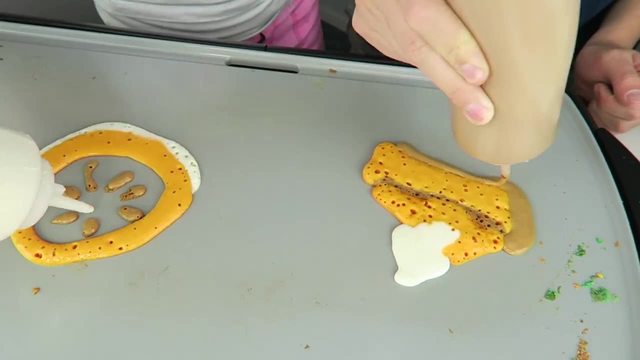 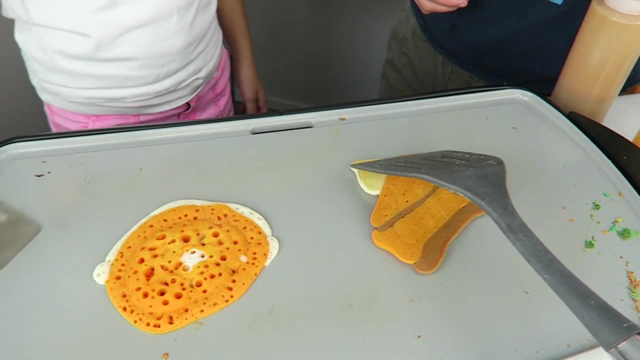 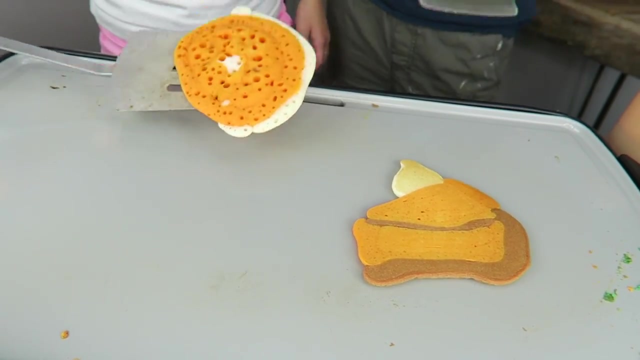 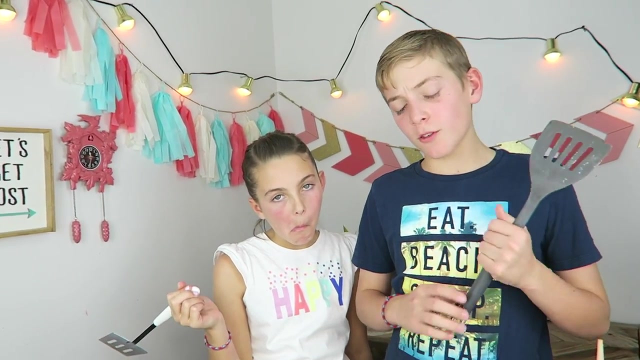 Okay, Time to flip them. I'm gonna flip it this way. Oh my gosh, That is pretty good. That looks amazing. Looks so amazing. Woo, Look at that, that's pretty good. So the thing that I was really going for was, like, I felt like this was super important, right here. 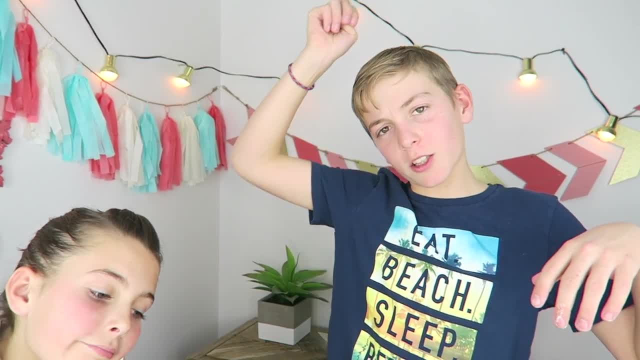 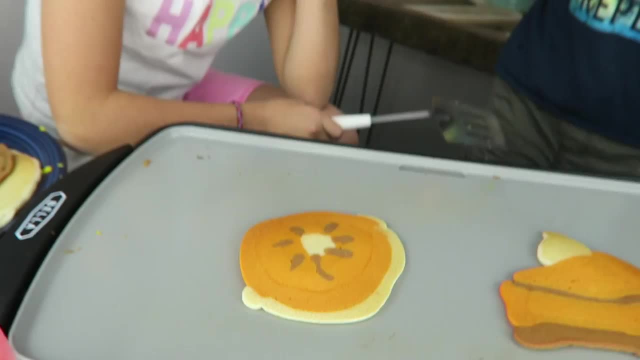 A lot of people like putting like the whipped cream sprinkles And the spiral on the top just to add a little bit more flavor. I went for a whole pie And I don't know what that white spot is but And then I did like the little lines in the pie. 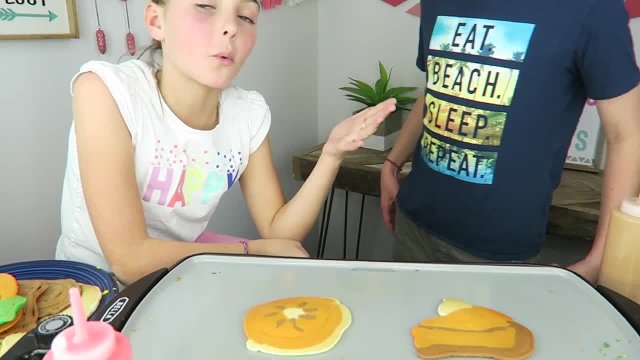 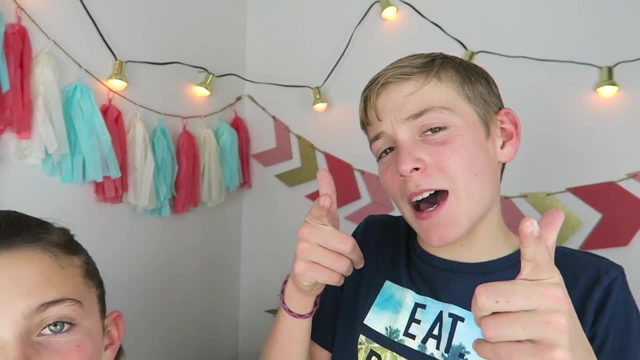 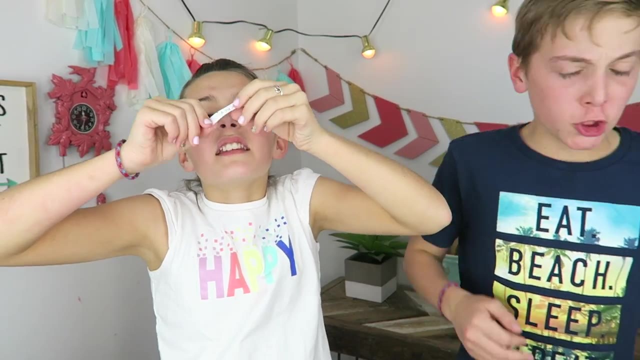 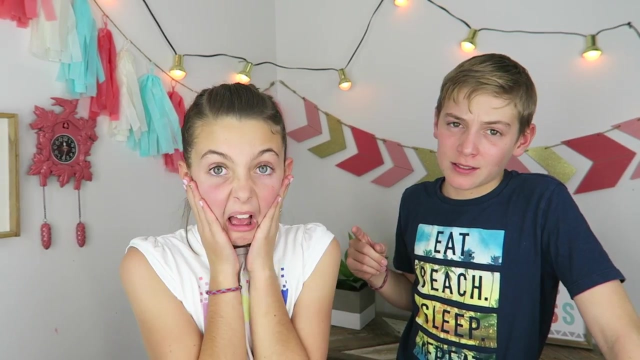 And then I tried to put like the pan with it, And then, of course, orange for the pumpkin pie. Alright, time to vote on the pumpkin pie. Me or Corbin, It's me. Turkey. This time it's a live turkey. That means like feathers and a beak and eyeballs. 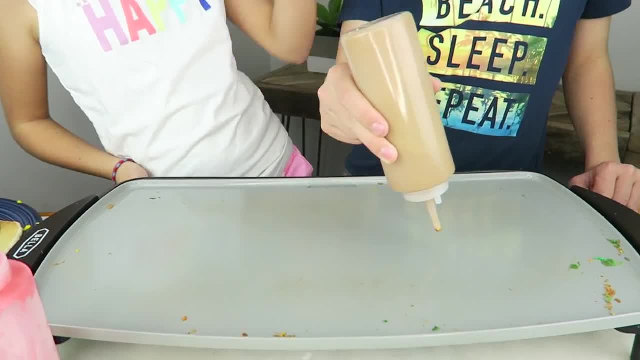 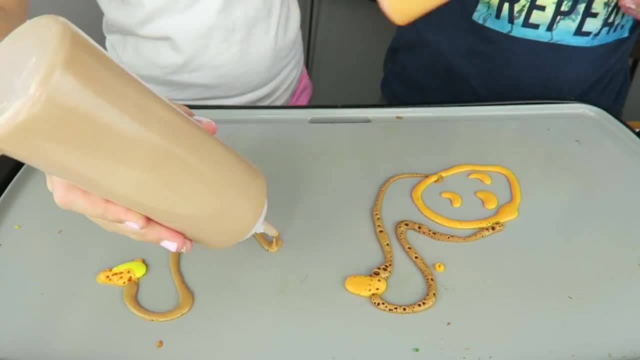 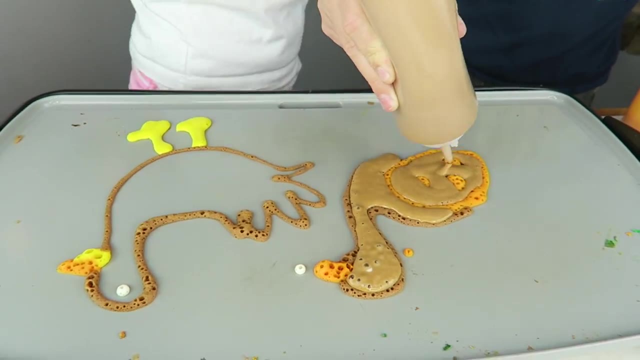 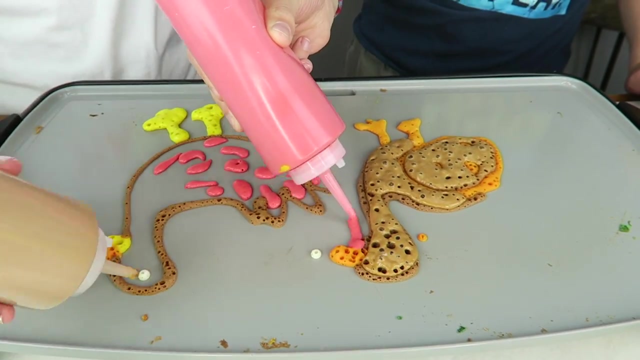 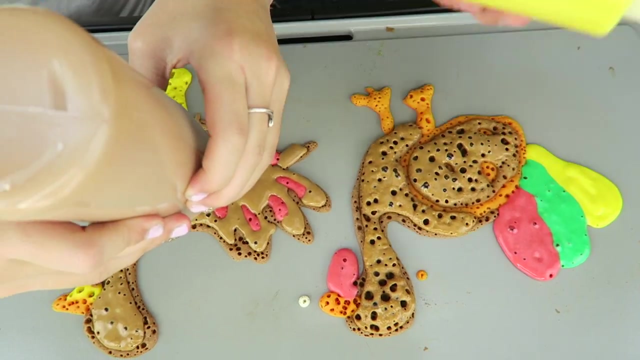 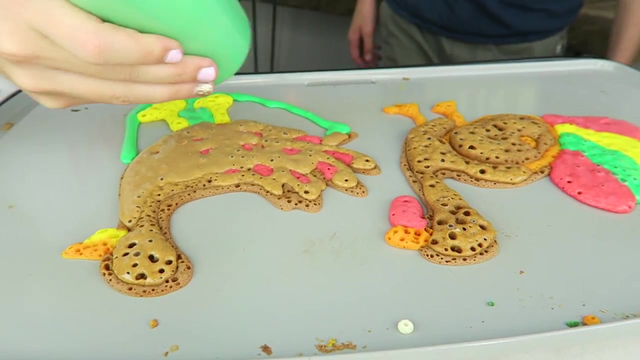 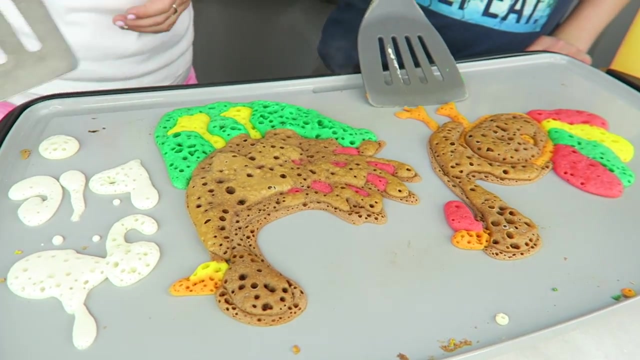 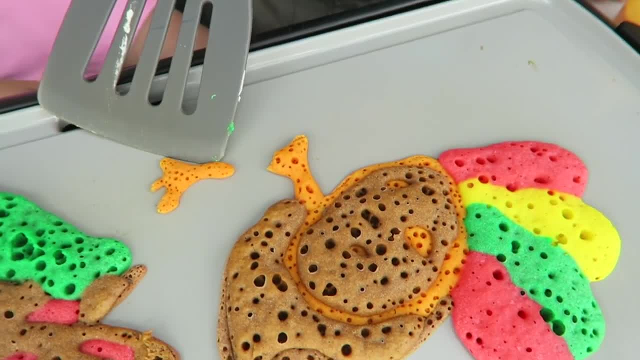 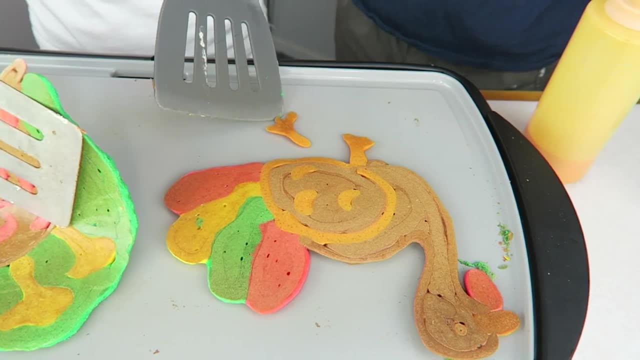 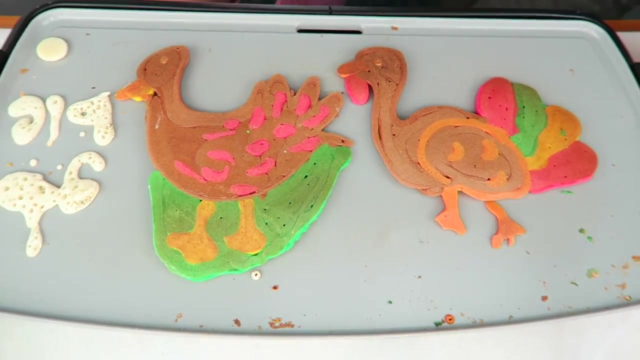 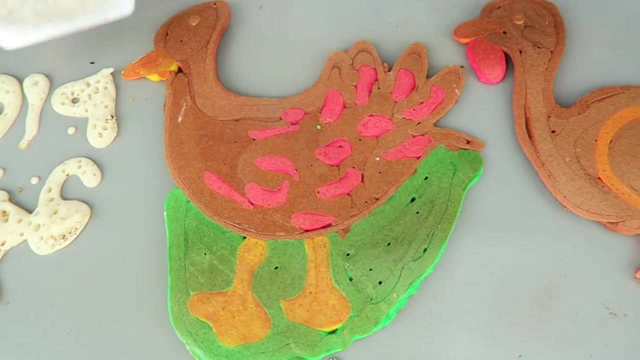 Guys, his leg came off. It's really bad. That's why I put mine in the grass. Poor little turkey. I did it, He died. I forgot, like the red thingy right there, It's double chin. And then I got the brown feathers, And then I put some red feathers in there, just for some color. 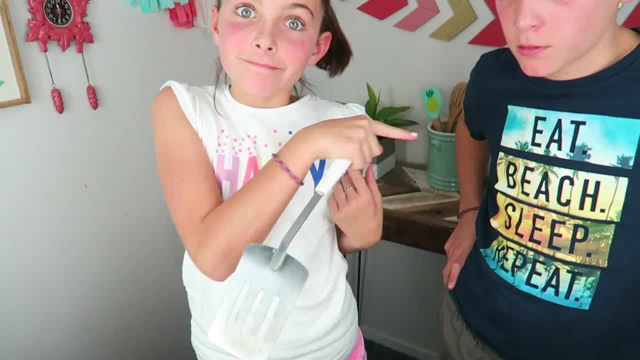 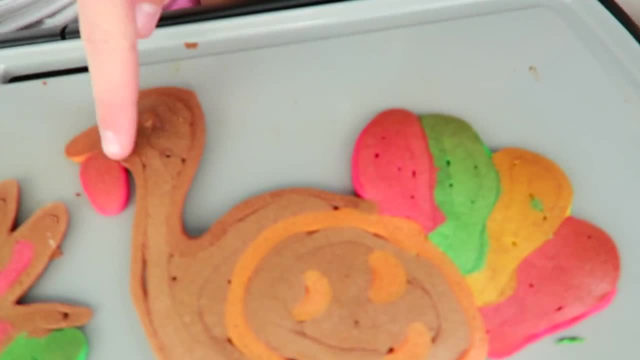 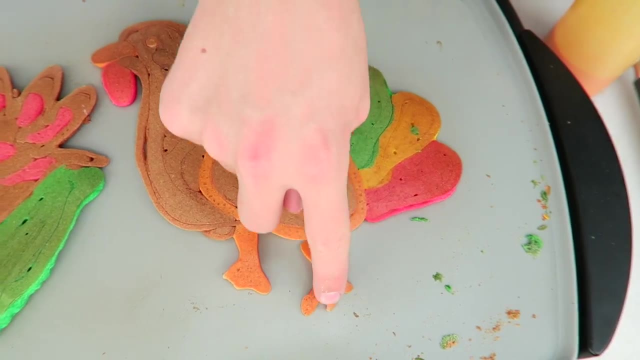 And then I put the legs in the grass so that the legs won't fall off. A little bit of something about mine. Unlike Ava, I did put the little gobble double chin thing on right there. I got his wing, His decapitated foot Decapitated. 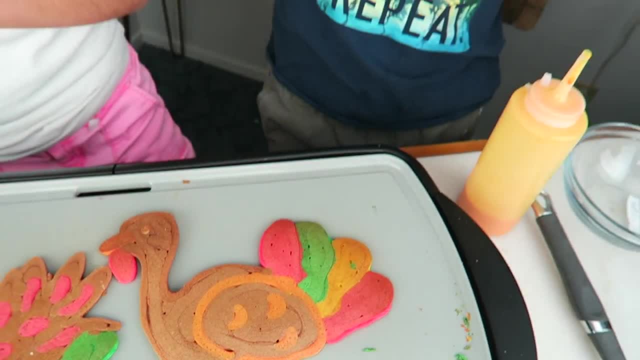 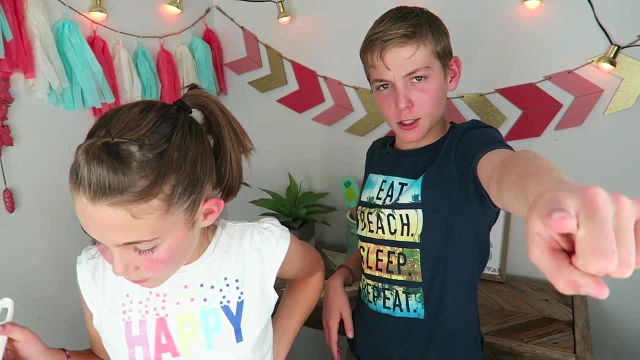 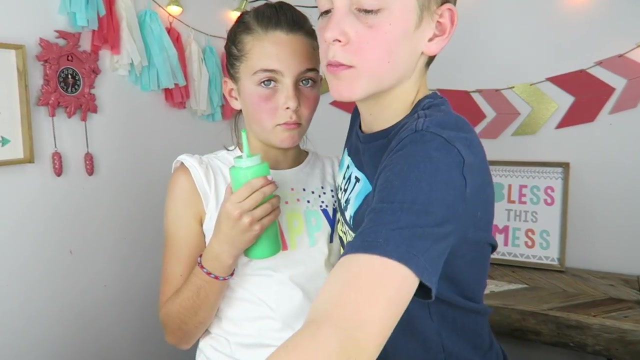 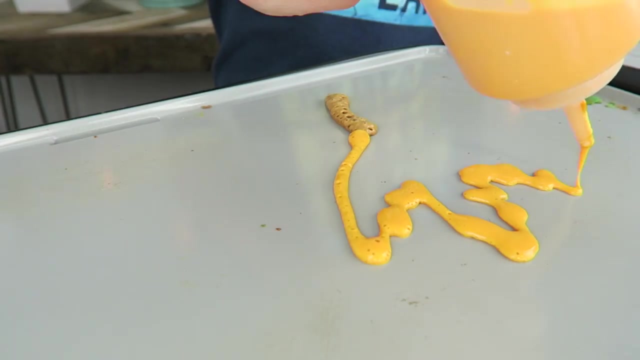 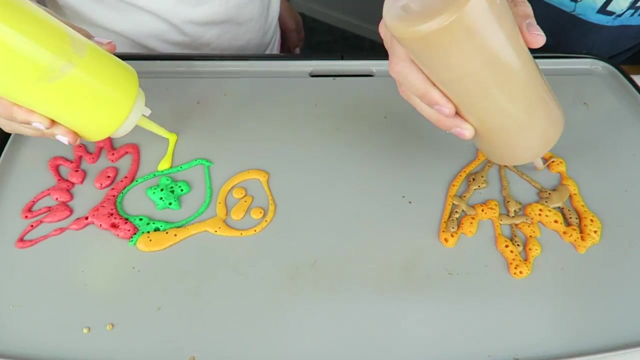 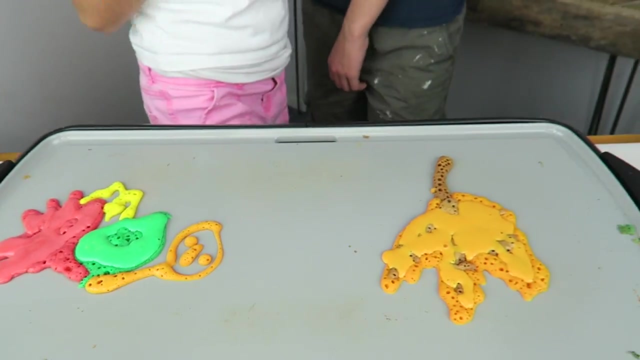 And then I also got the beautiful colorful feathers that a turkey has. Now go vote. I want you to vote for me, So the last one that we're going to do right now is a fall leaf. Oh yeah, So Mine, Don't tell me that doesn't say delicious to you. 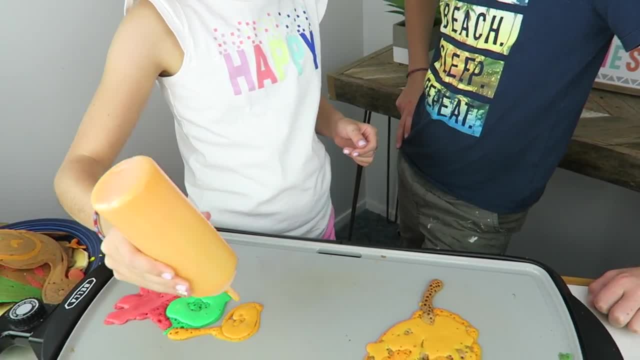 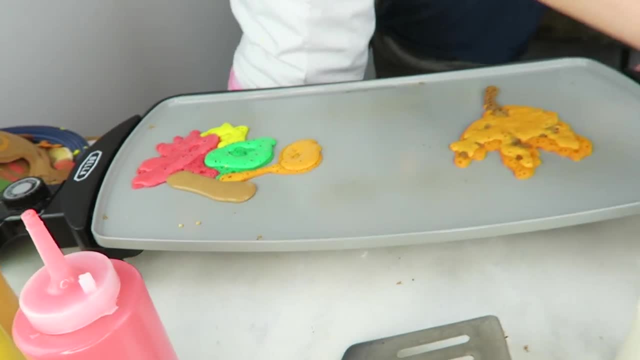 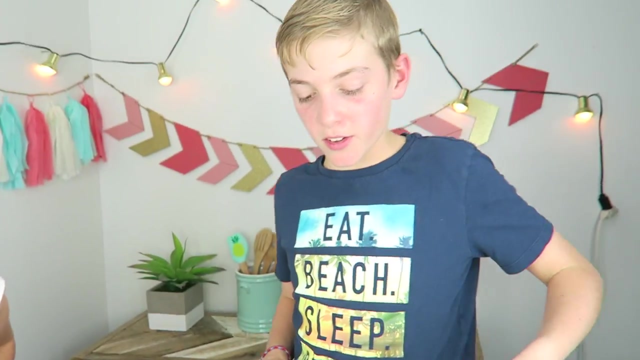 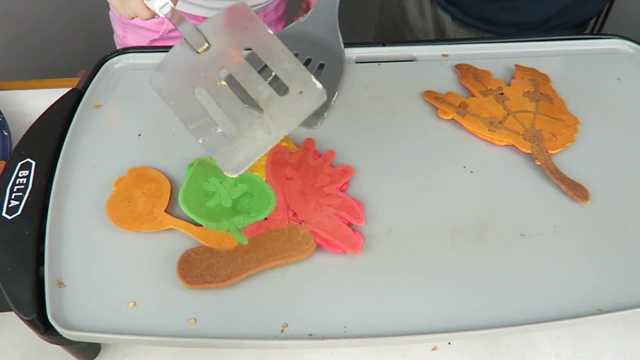 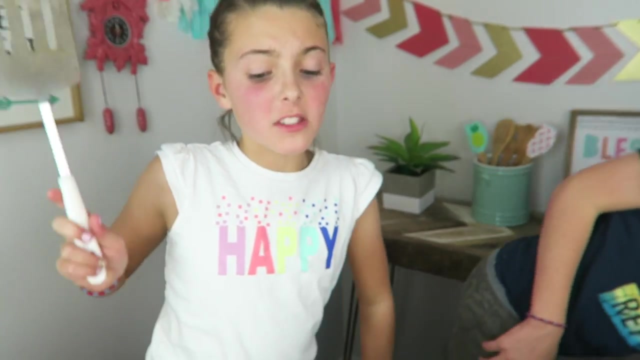 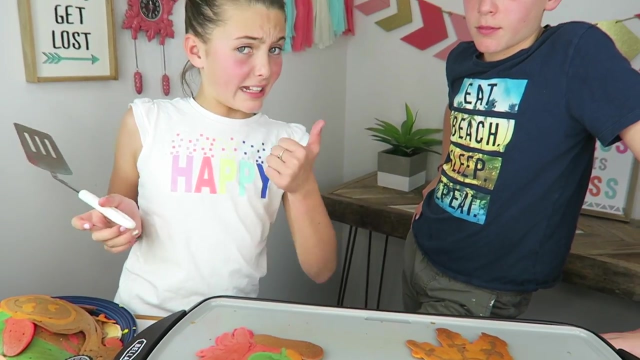 Okay, here is my fall leaf. Look at that, goodness. I surprise even myself sometimes. Bow, Okay, so a little tour of mine. I put the red leaves, the yellow leaves, the green leaves and even the orange leaves. That one just looks like a pumpkin hanging from a tree. but that's okay. 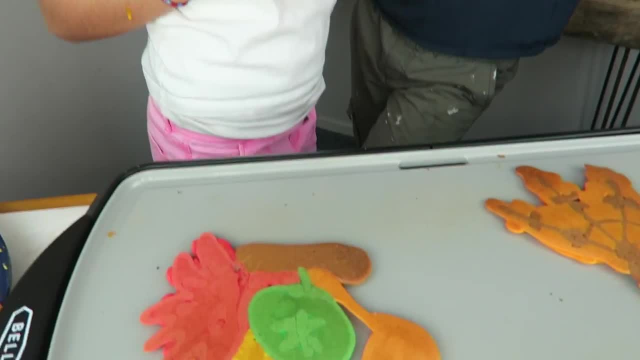 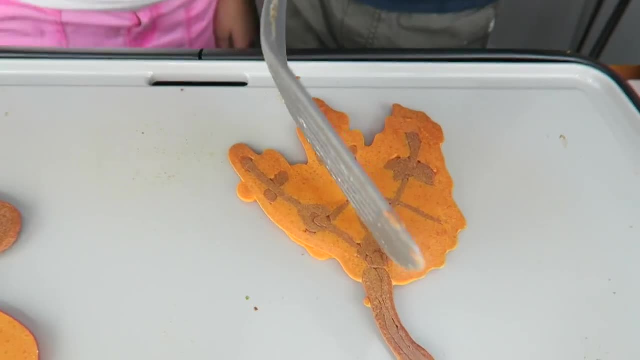 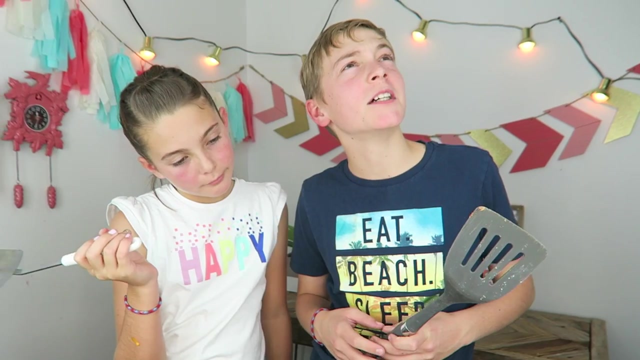 And then I put the brown sticker here, so it's like hanging off of a tree. So a little something about mine. I went into a little bit more detail. I have the connecting point to the leaf. It stabilizes it and allows it to grow Prosper. Okay, that was our last one. 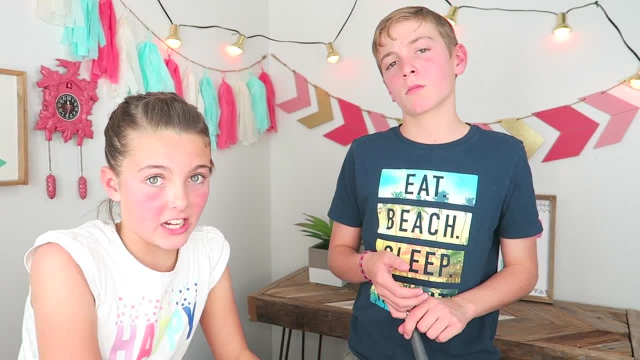 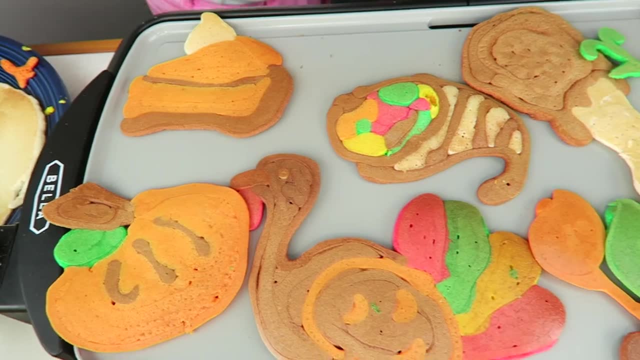 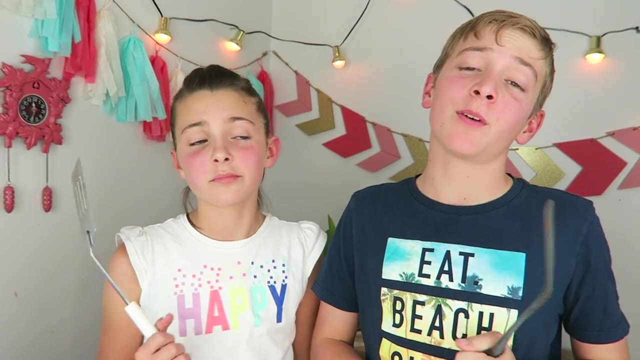 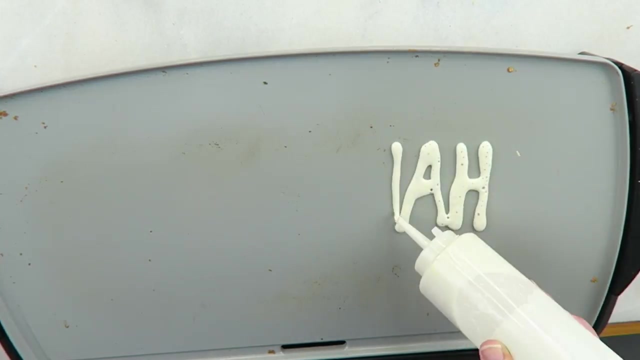 Time to vote. Who won the whole pancake? challenge Me or Corbin? Comment down below: Alright, you guys. thank you so much for watching this video. Hope you have a very happy Thanksgiving. We'll see you guys next time. Bye, Thanks for watching. 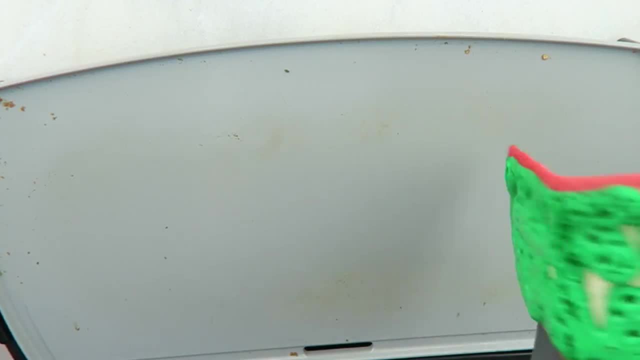 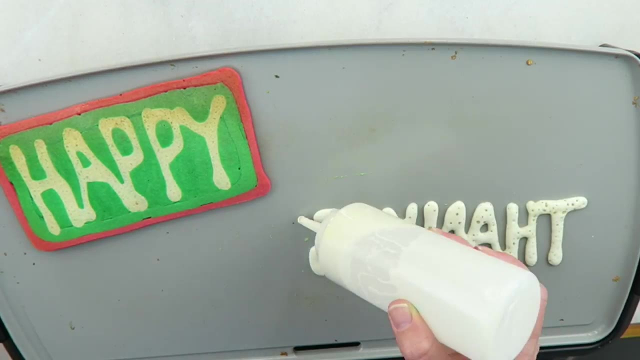 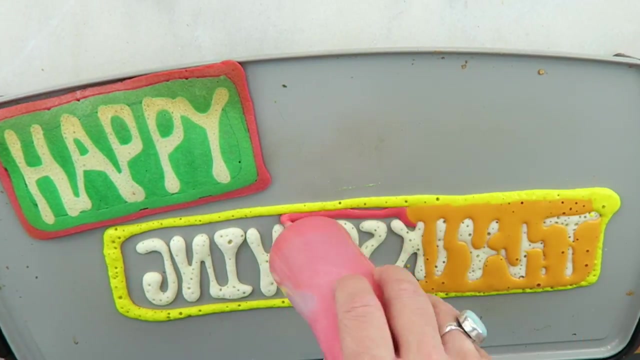 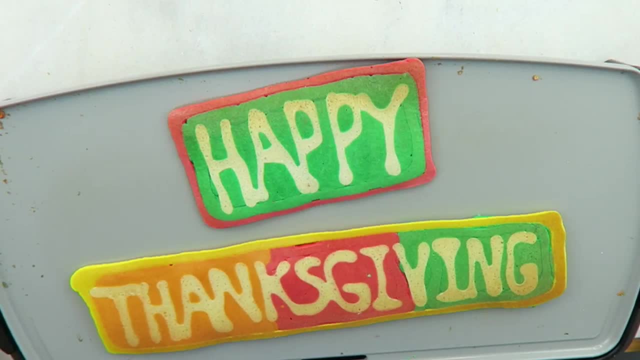 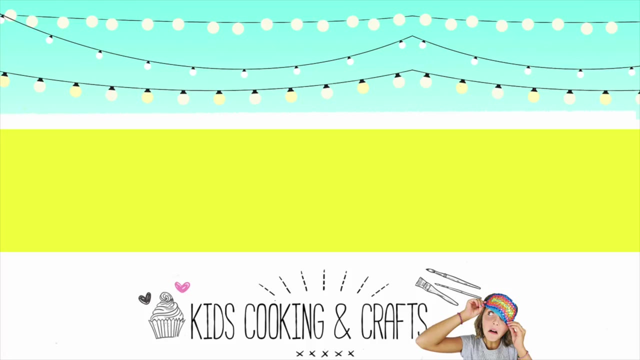